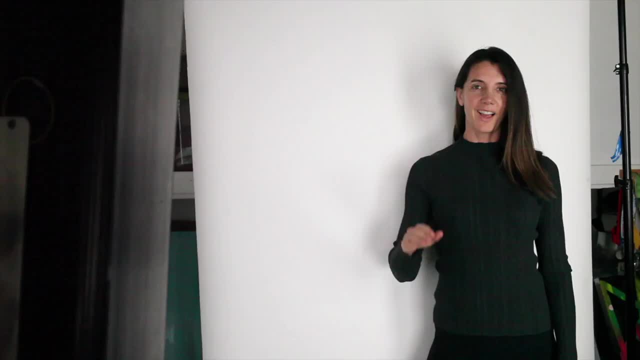 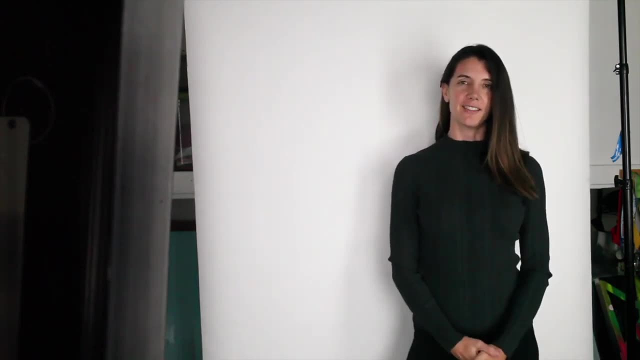 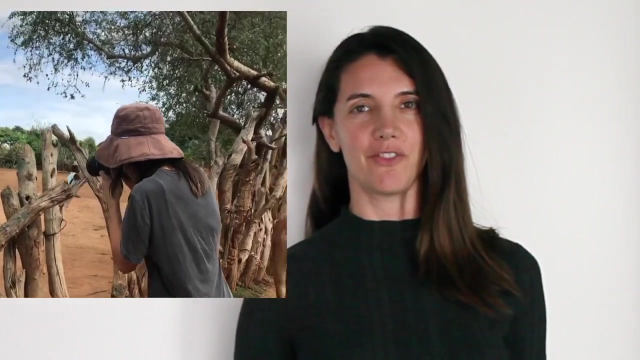 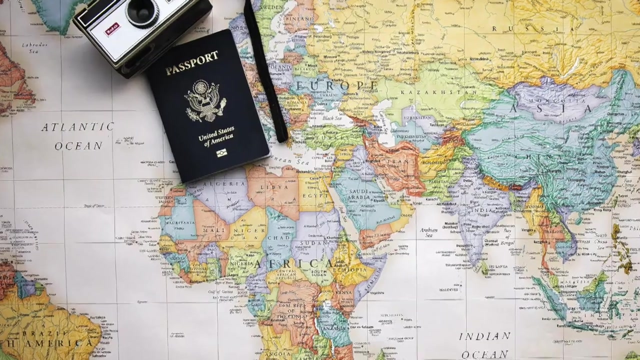 Hi, my name is Nadia Tyson and I am a documentary, fine art and headshot photographer. A little bit about me. I started photographing around 20 years ago when I got my very first film camera. At the time I was about 18 and I was traveling quite a bit and what really pulled? 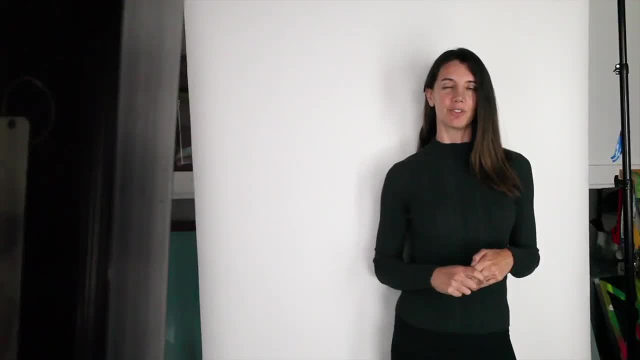 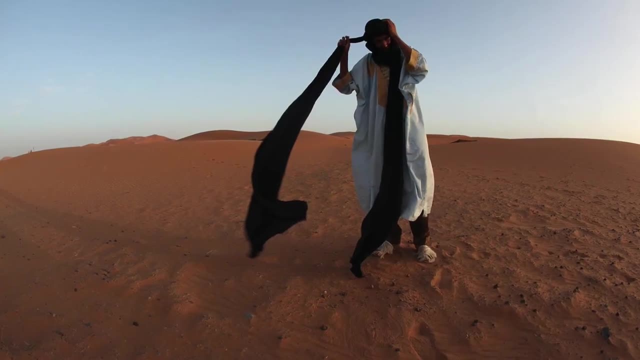 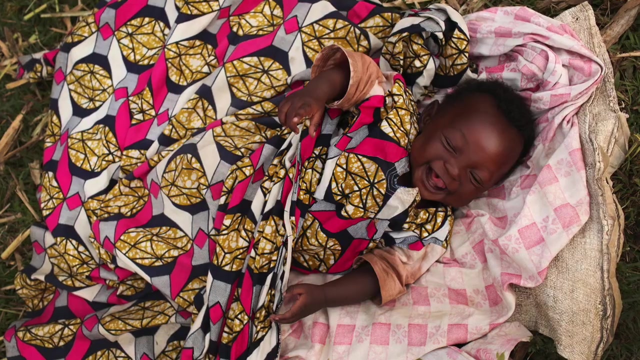 me into photography was being able to take photos of anything that I thought that really pulled me in and captured my attention, and being able to share those photos, once I got back home, to my friends and family, And so they were able to understand what I was seeing. 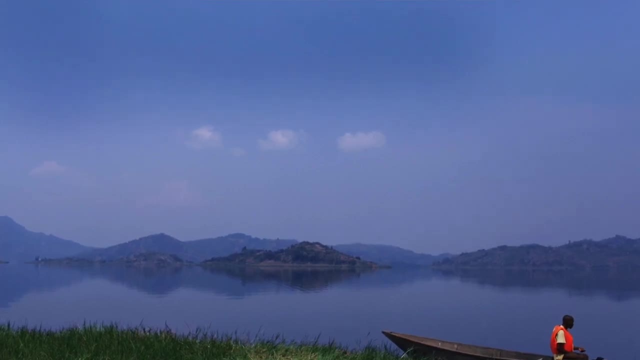 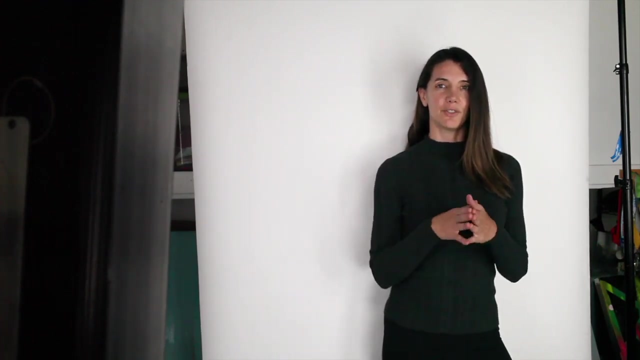 through what I took and my vision of how I saw things, And so since then my passion grew. I studied photography for a little bit, and I really don't go deep into learning more about documentary and portrait photography, So that's what I specialize in now. I have photographed for a number of magazines, a couple books had. 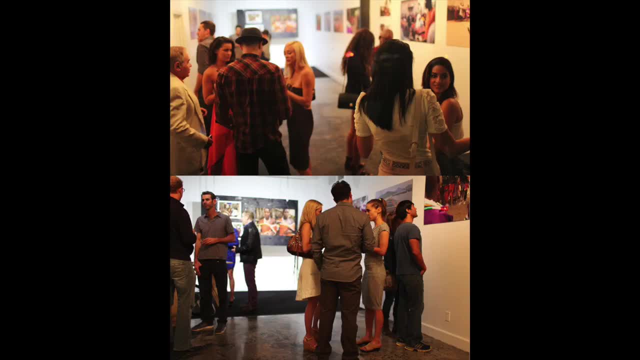 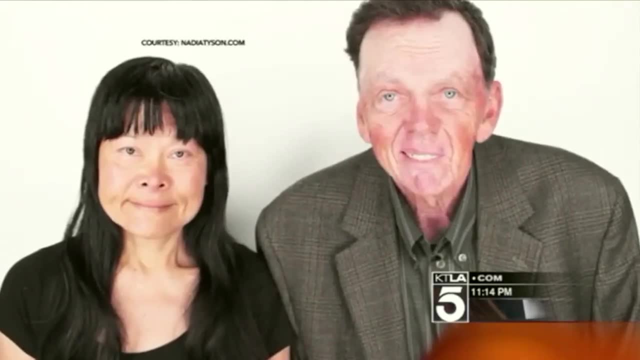 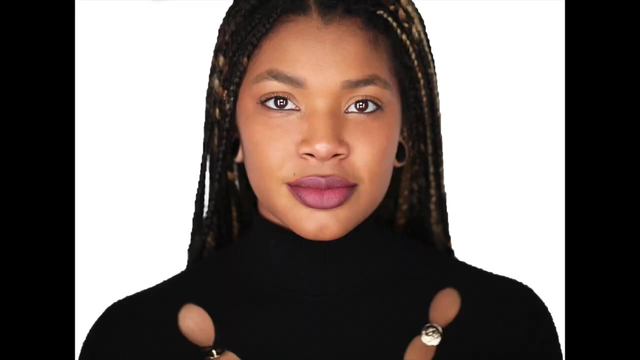 a few shows, and I've also had the opportunity to photograph for a philanthropist on an amazing photo project we did here in LA. On top of that, I have a small headshot business and that has allowed me to photograph a range of people all the way from actors, lawyers, doctors, social media. 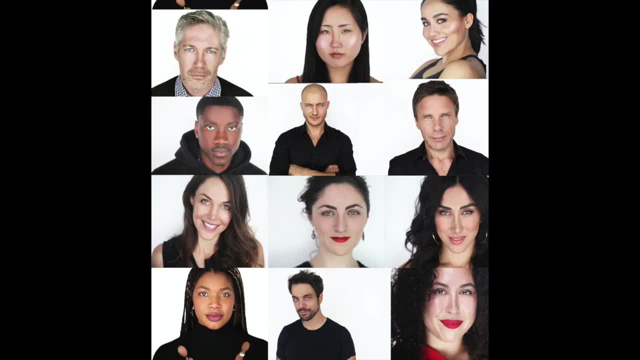 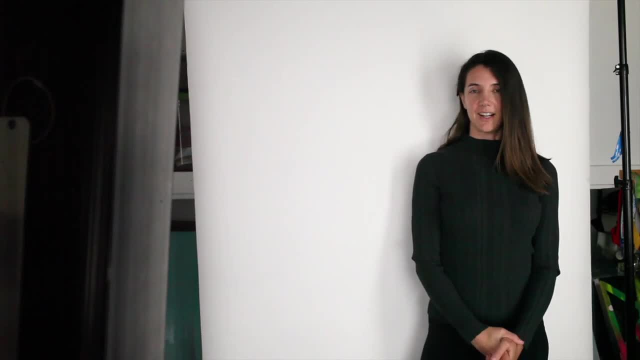 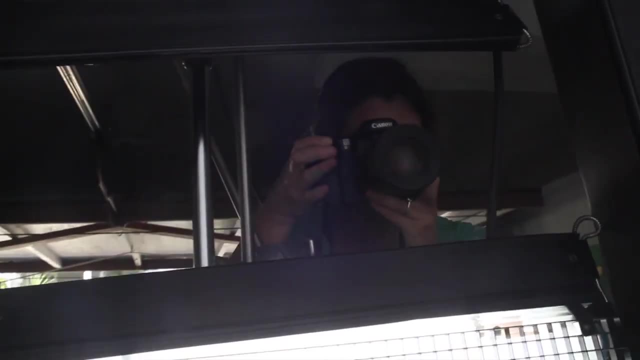 influencers, models and all the other types, And this is even the background I use when I photograph for my headshot business and this is the lighting I use, And that has also allowed me to photograph several corporate business company headshots, which is super. 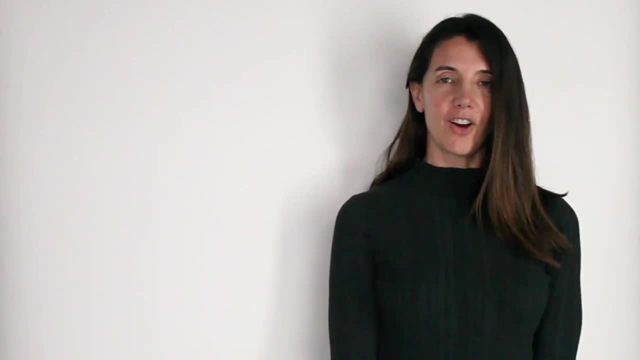 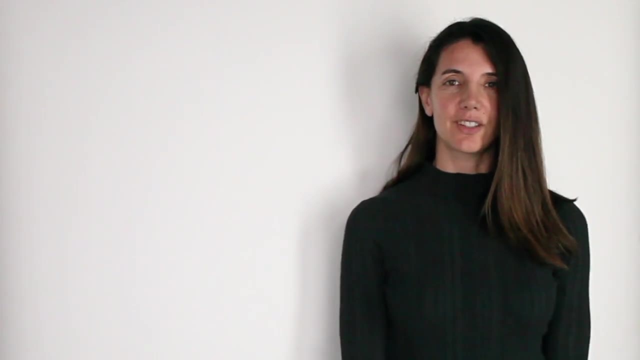 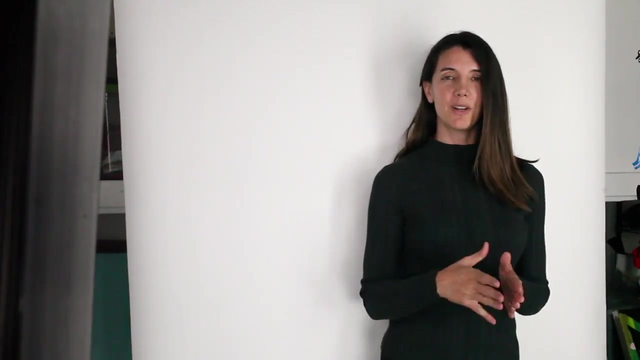 fun for me to do. And finally, I also teach digital photography to middle schoolers at a school in Los Angeles, So a lot of the lessons that I teach here are very similar to what I teach in that class. This class is composed of two main topics. The first one is learning how to use your